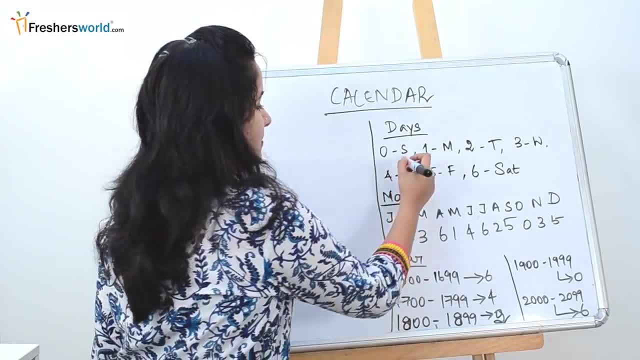 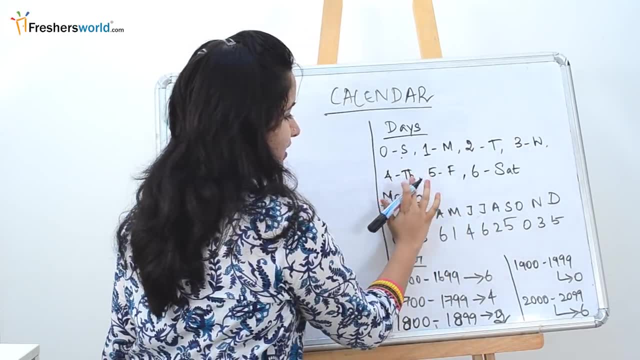 So in days we are going to number each day. So we are going to start from Sunday, So we are going to put 0 for Sunday, 1 for Monday, 2 for Tuesday, 3 for Wednesday, 4 for Thursday, 5 for Friday and 6 for Saturday. 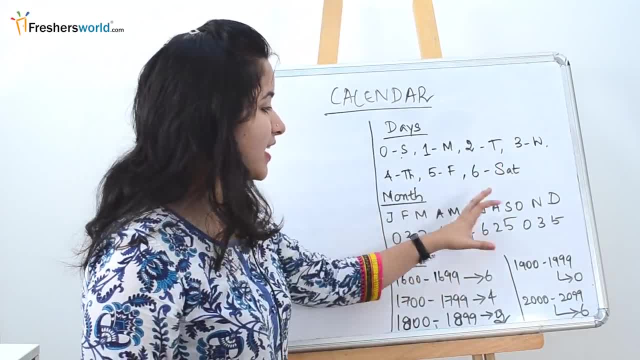 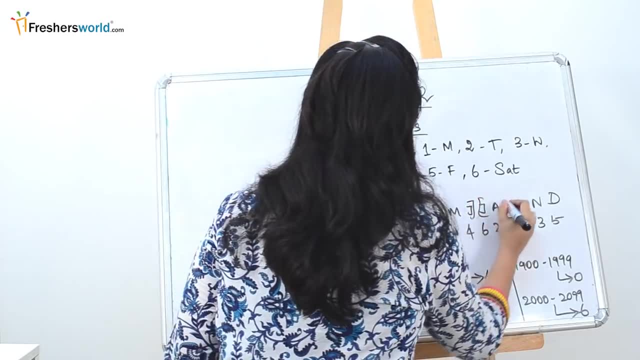 Similarly, from month, from Jan to December. we are going to code each and every month with a number. So how to remember this number? Remember it like this: So split it into 3 months, So the first 3 and the last 3.. 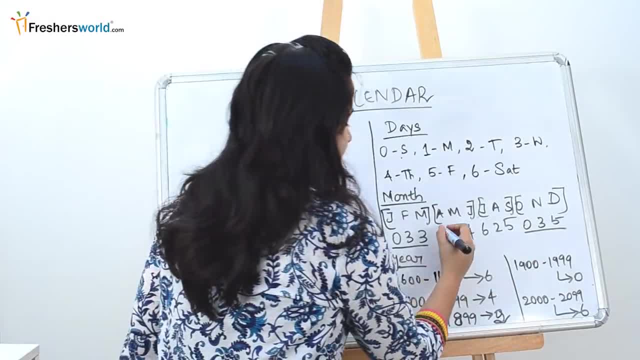 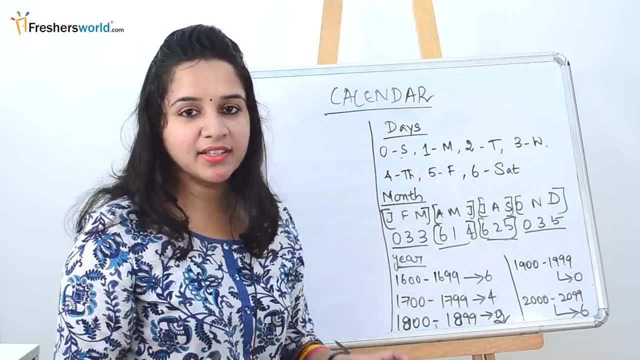 It is nothing but 033, 035.. And the middle 2, you can remember it comes in 6, which is 614 and 625.. So first, when you see the answer rough sheet, you can write from Jan to December. 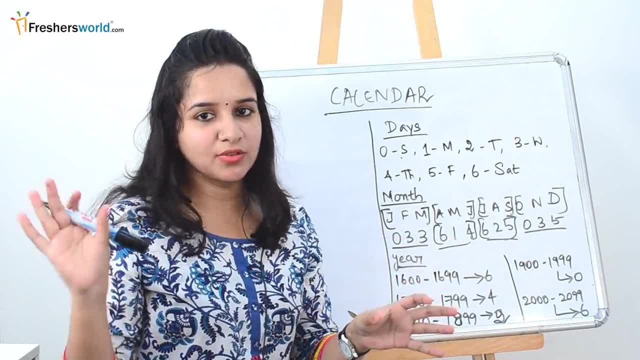 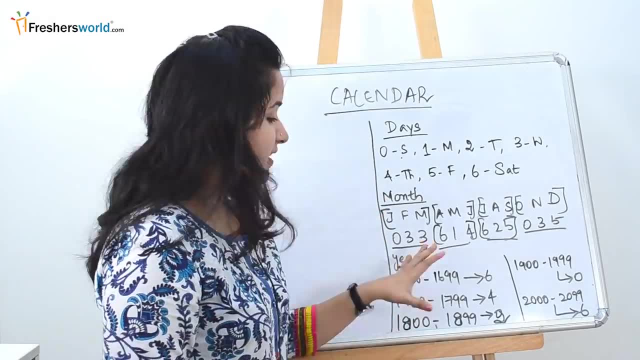 Then first fill the first 3 and the last 3 as 033 and 035. Then in between you can fill it as 614 and 625.. That's how you can remember it as a month, Then for the year- these are the various years that they generally ask in all the type of questions. 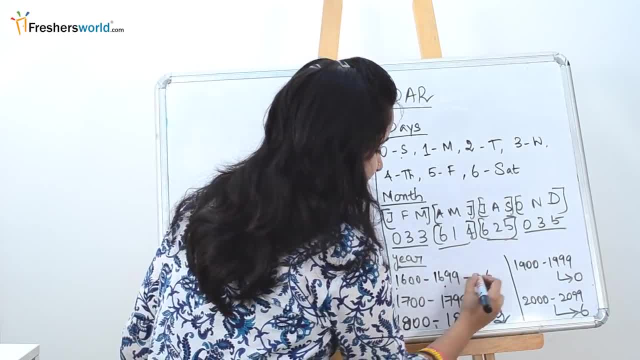 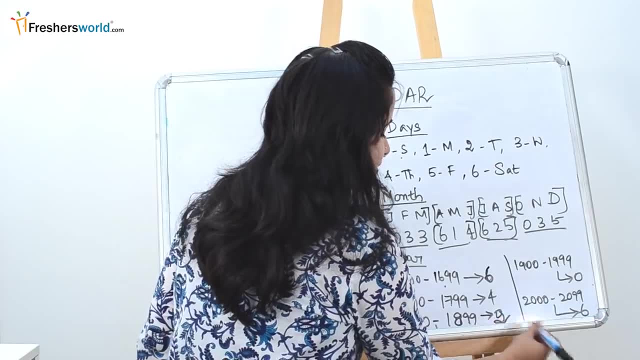 So from 1600 to 1699, we code it as 6.. From 1700 to 1799, we code it as 4.. 1800 to 1899, code it as 2.. How to remember this? 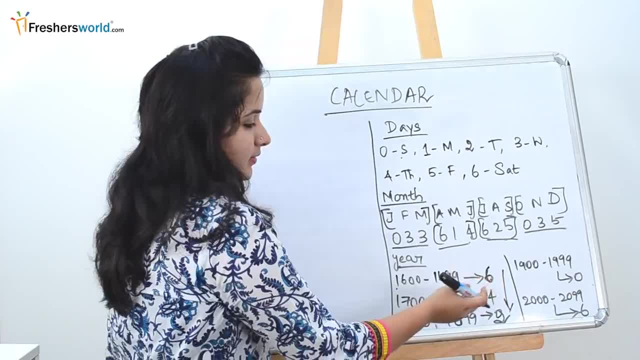 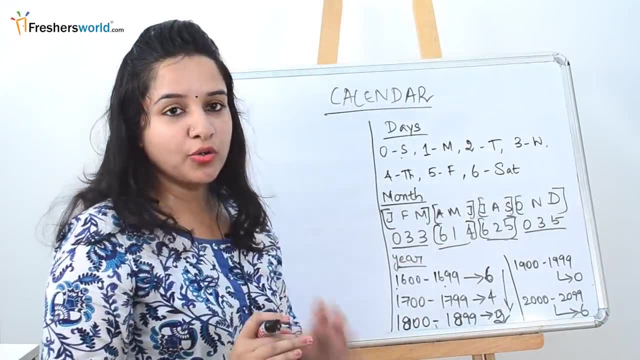 Go in the descending order From 6, 4, 2.. For 1900 to 1999, it is 0. And 2000 to 2099, it is 6.. So how do we do it? 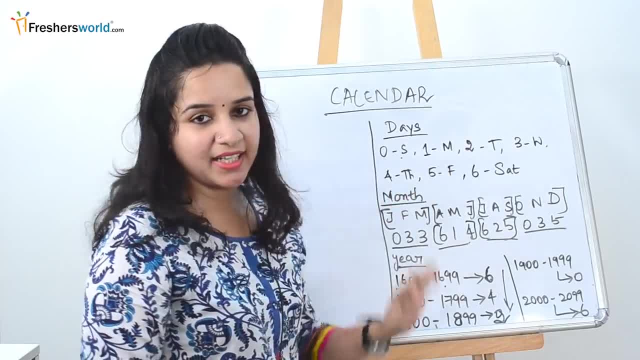 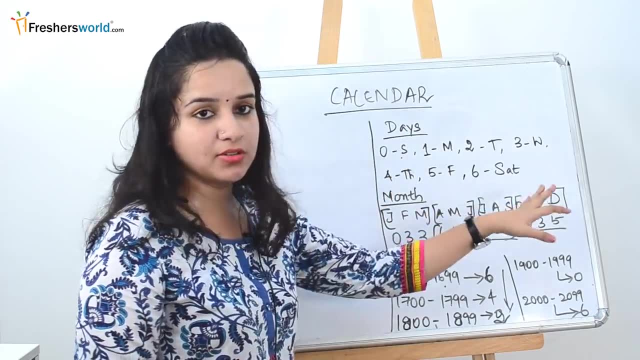 From days from Sunday we actually code it till Saturday, So 0 to 6.. For month, remember the first 3 and last 3.. Then fill the middle from Jan to December. Similarly, for year, we are starting from 1600 till 2099.. 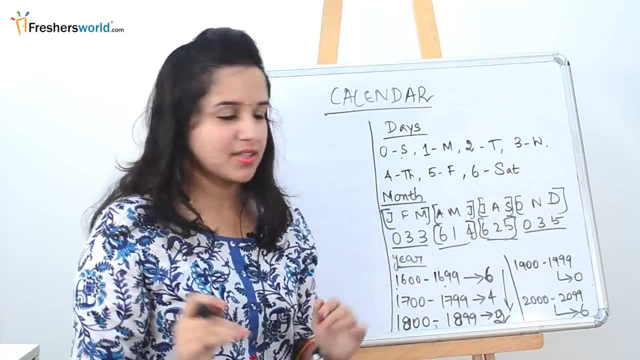 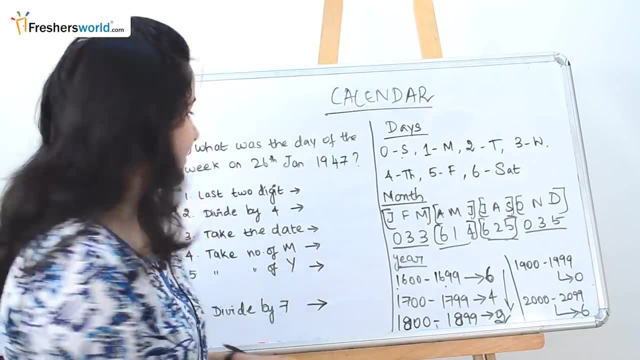 How do we do it? 642 and 06.. So remember these codes for solving the calendar problem. So let's get started with the simple question now. Okay, the first question that they have given is: What was the day of the week on 26 Jan 1947?? 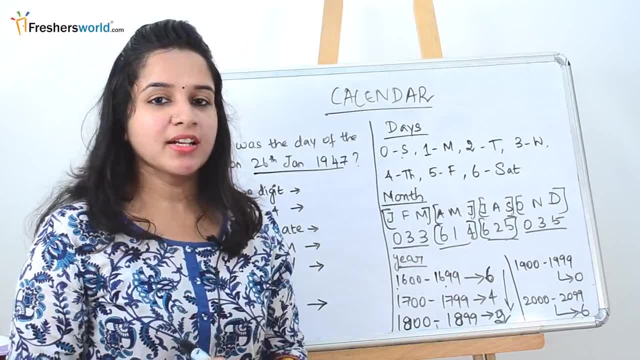 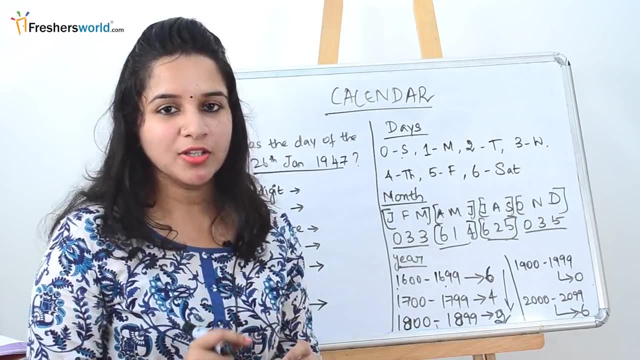 So this is the question that they have given. So there are basic 6 steps One need to follow to answer this question. Those are very simple steps. So once you understand the concept of these 6 steps, you can solve it within 15 seconds. 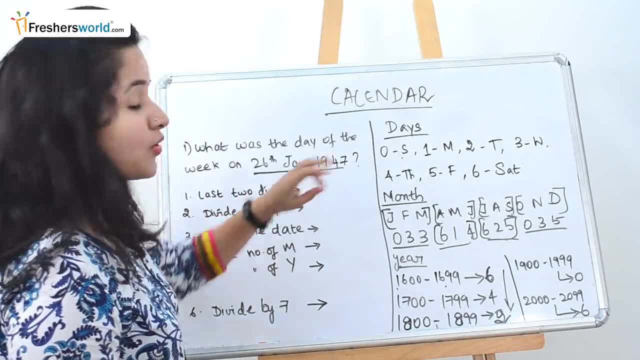 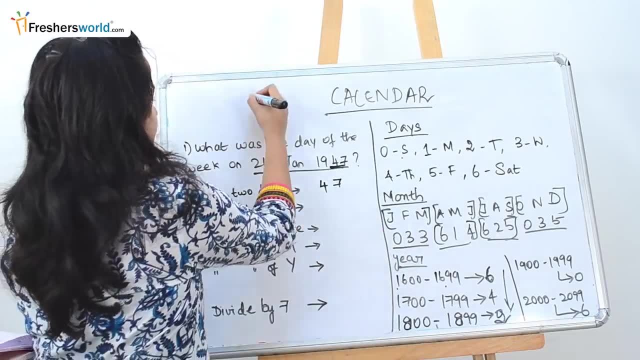 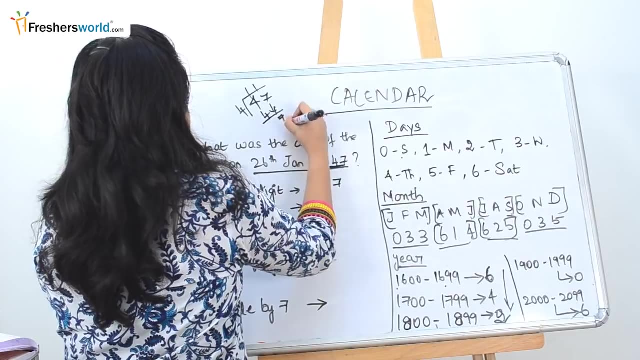 So first you have to take the last 2 digit of the year. So what is the last 2 digit of the year? 47. So next divide it by 4.. You have to divide 47 by 4.. 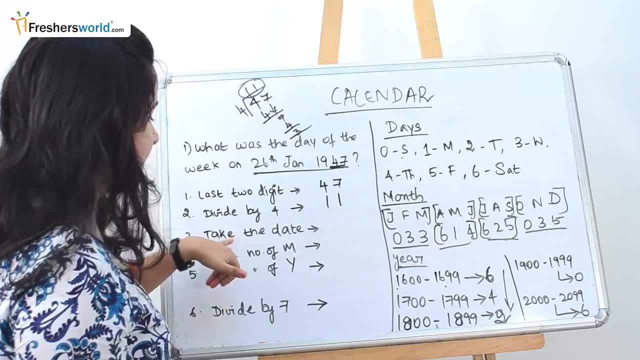 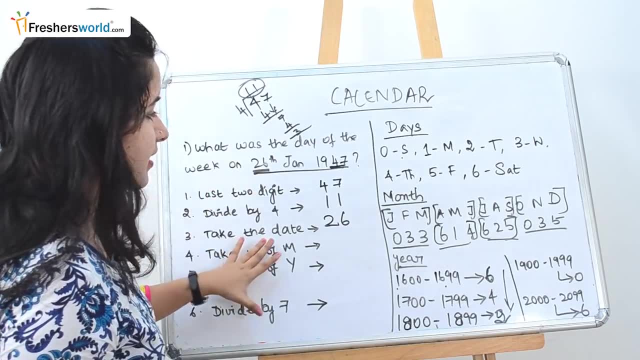 So take your quotient, Next take the date. So date is nothing but 26th. Next take the number of the month. So from here these things will come into place. So what is the number of the month? 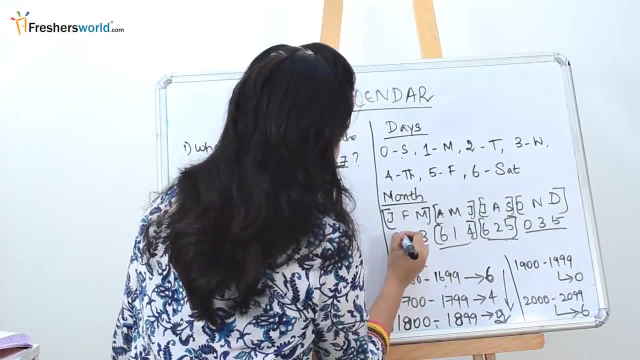 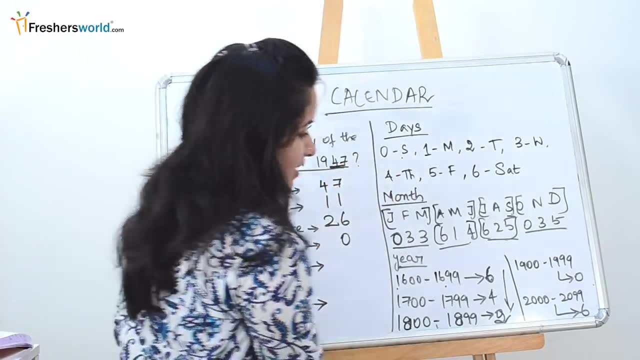 What is the month? Jan? So Jan is nothing but 0. So we take 0 here. Next take the number of the year. So year is nothing but 1947.. So 1900 to 1999, which is also 0 here. 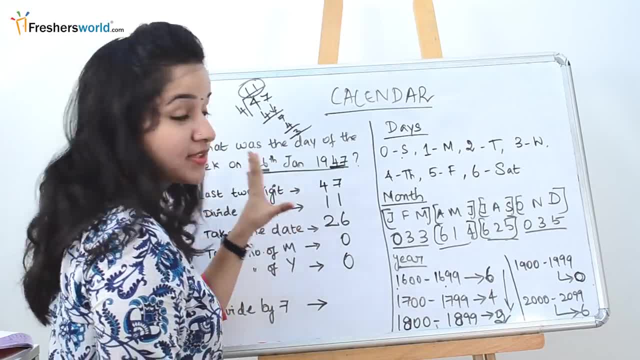 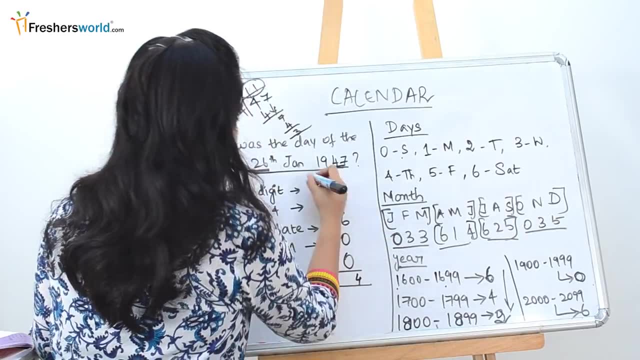 So we take it as 0.. So now you add these numbers, These first 5 steps: 7 plus 1, 8.. 8 plus 4, 8 plus 6 is 41.. 5, 8.. 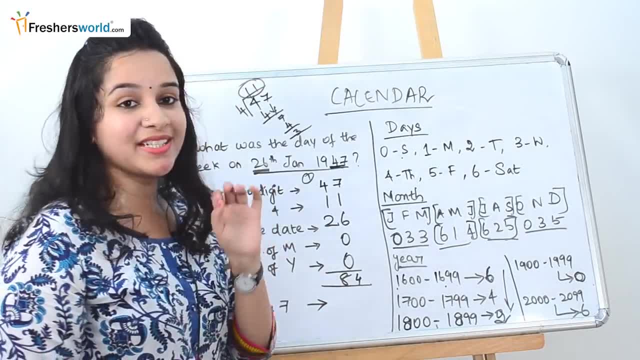 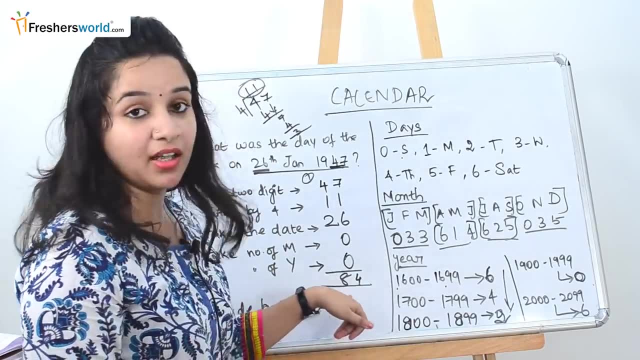 84.. So your total is 84.. What is the question? What is the day of the week? So how many days in a week? 7 days, So you are dividing 84 by 7.. We know that 12 sevens are 84.. 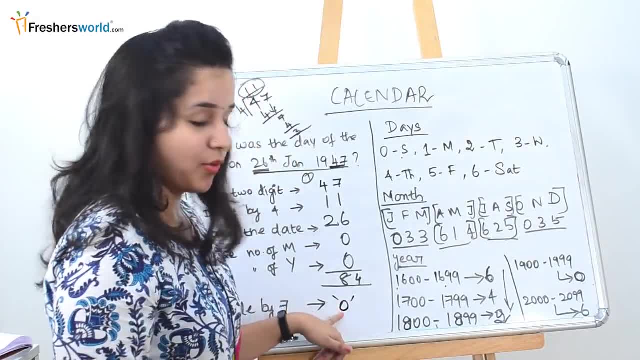 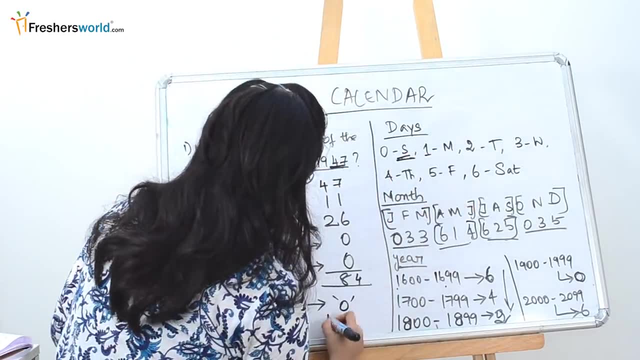 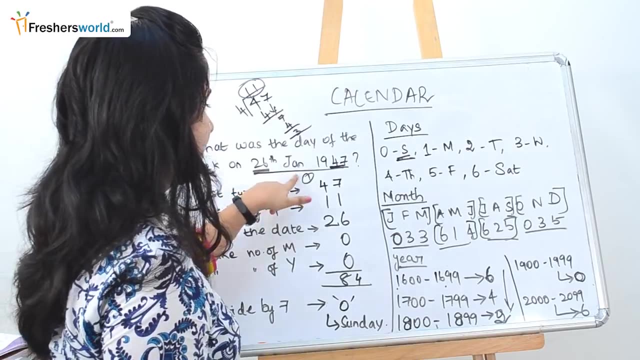 So you will obviously get the reminder as 0. So you have to take reminder here, So 0. So what is it corresponding to? 0 is nothing but 0. And Sunday here. So what was the day of the week on 26th Jan 1947 is nothing but Sunday. 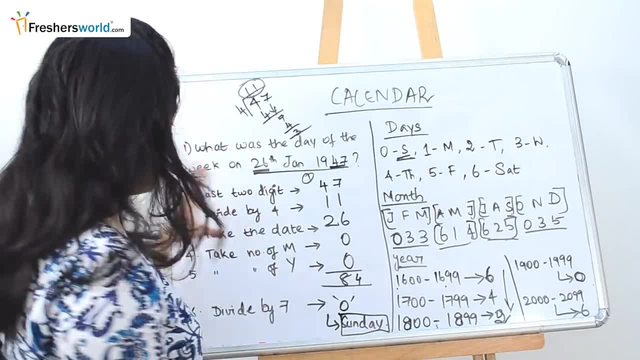 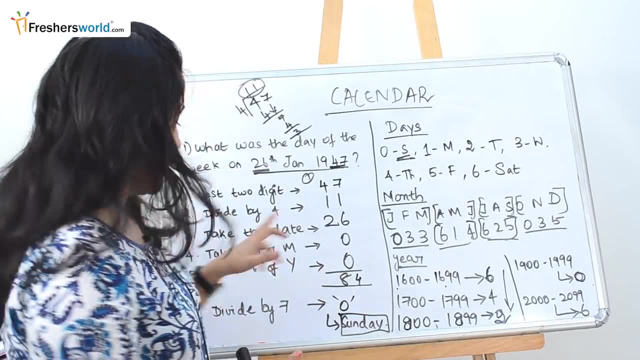 So, in this question, what you need to know for the first 5 steps: First you have to take the first 2 digits divided by 4.. Next, you have to take the date. Next, you have to take the number corresponding to month, number corresponding to year. 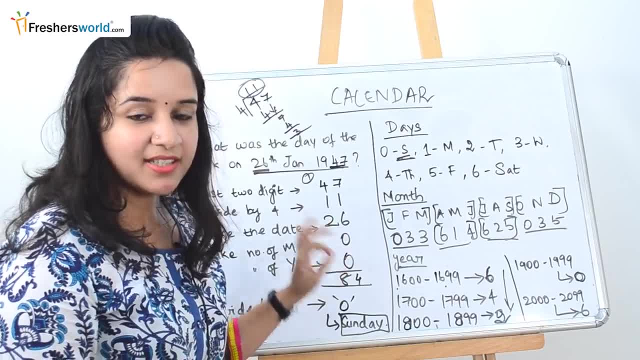 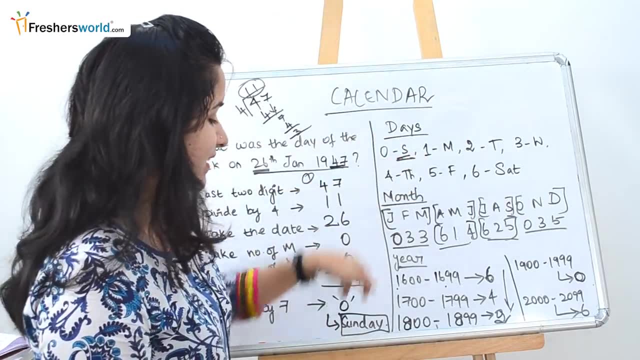 Once you get the first 5, add it. Then they are asking for the day, So you will divide it by 7.. The reminder of it: nothing but corresponds to the number code of the days, So you can directly write it. 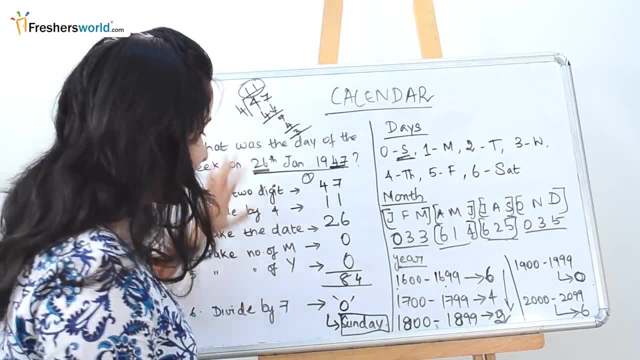 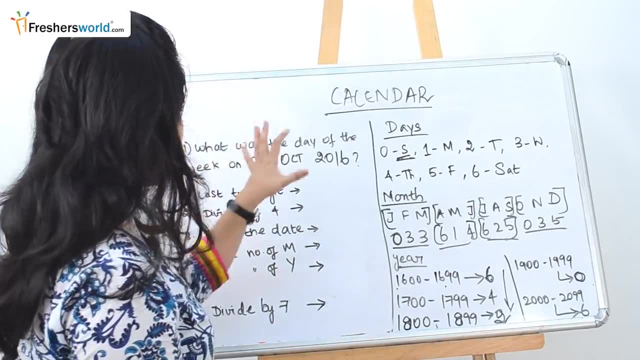 So initially it will be really tough, But once you understand the 6 steps really easily, you can finish off the sum. Let's solve another example. So the next question is: what was the day of the week for 5th October 2016??